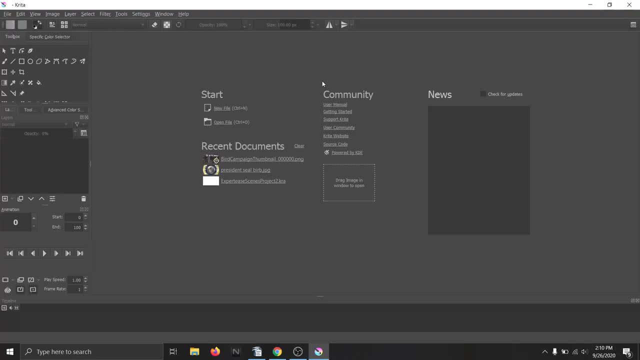 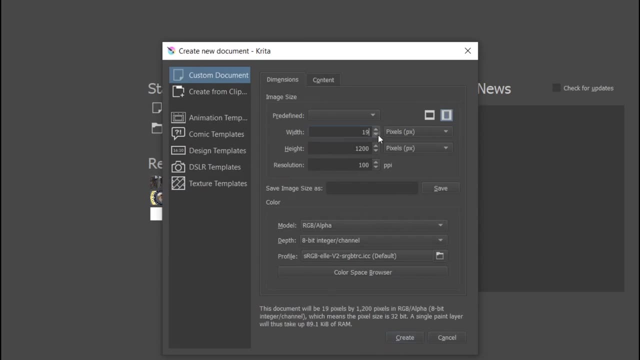 Creating a Project. Once you see the opening screen, click on New File. It will bring up a little pop-up window where you can choose a style, Size, resolution as well as the color format For YouTube. you will want to set it to 1920x1080 pixels. 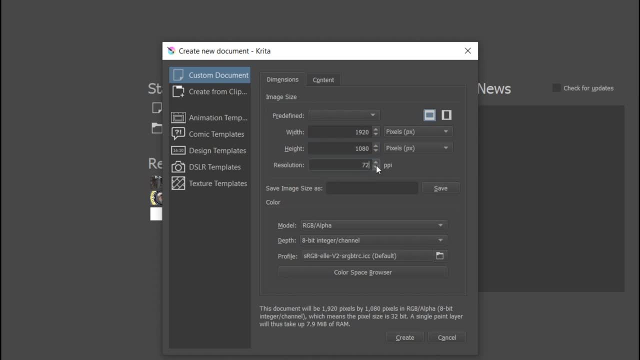 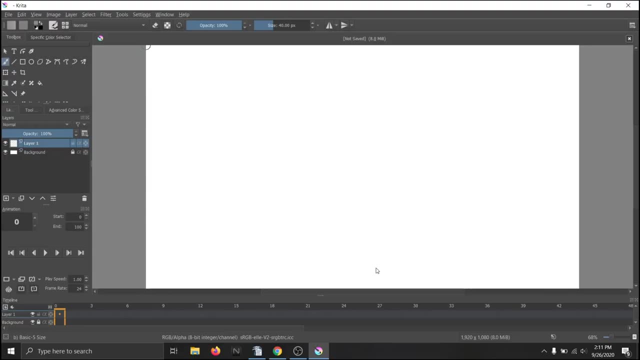 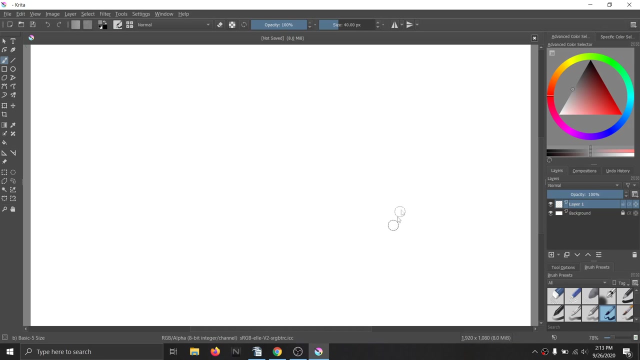 The resolution doesn't really matter unless you plan on printing it out on a poster, so 72 will work just fine. Once you're satisfied with your settings, click on Create, which will then bring up your default workstation and an empty project. To get to the animation workstation, go to the top right corner and hit this little drop-down menu button. 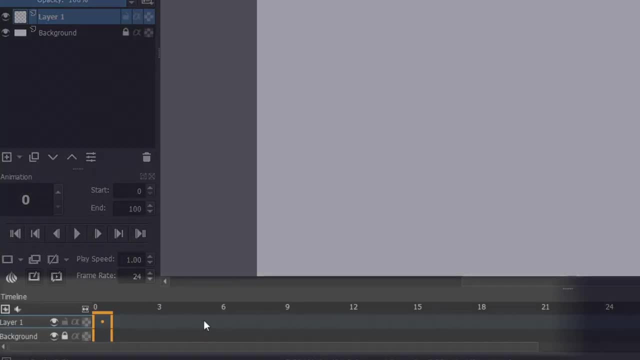 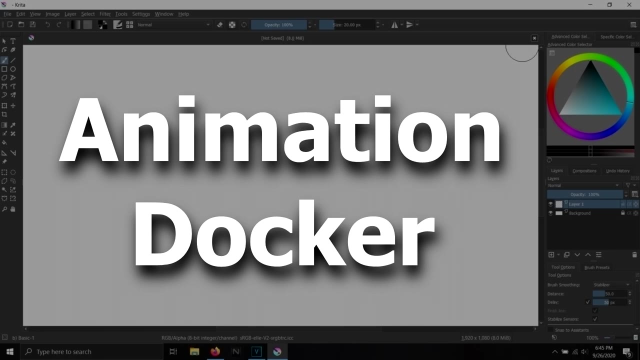 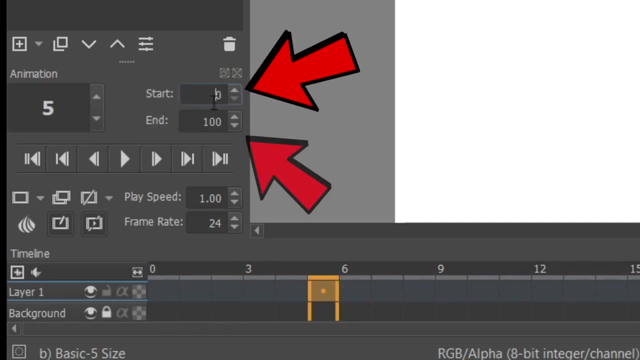 And select the animation workstation. This will bring up your timeline and animation dockers, which are the two dockers you'll need to animate. Now let me quickly explain the animation docker. The animation docker shows you the current position you are on in the timeline, along with the starting and ending frames of your animation. 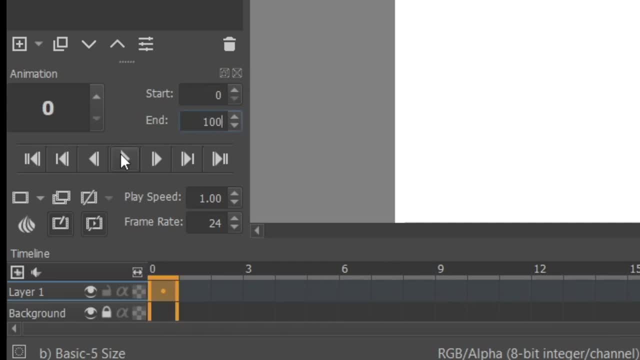 Basically how long it is, And these buttons can be used to play your animation, skip a frame in your animation and skip to the beginning or end. The next button is Add Blank Frame which, as you can see, is used by clicking on it and having your cursor at the desired position on the timeline. 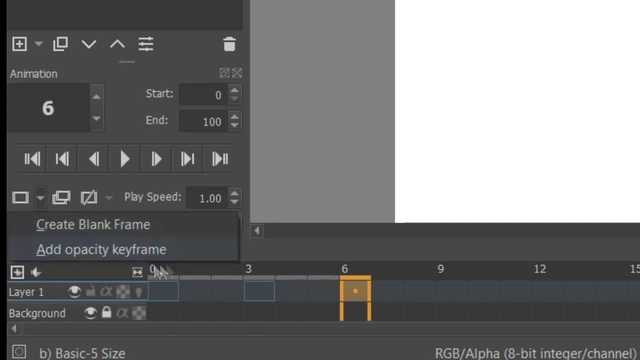 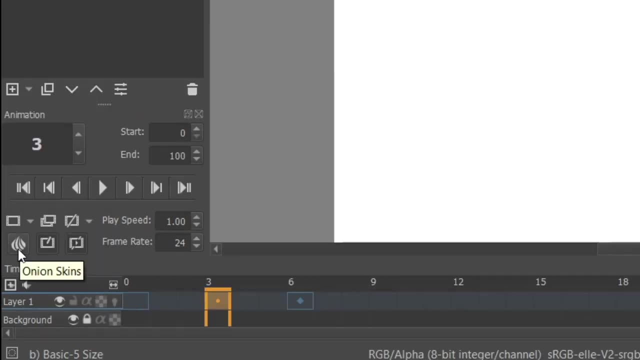 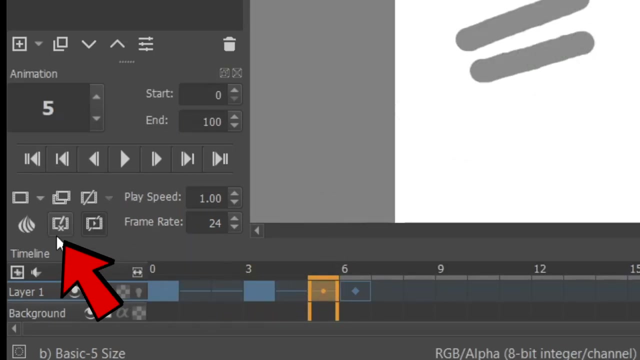 You can also add an opacity keyframe using the little down arrow next to the button. The remaining buttons are: Duplicate Frame- Remove Frame. Onionskin, which brings up the settings. Auto Frame Mode, which creates a new frame every time you draw on a new keyframe on the timeline. 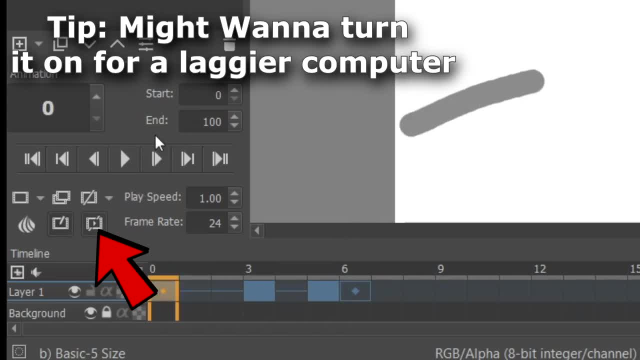 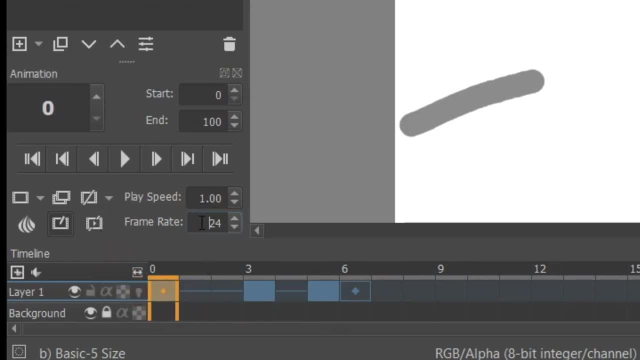 and Drop Frames, which drops frames during the playback if your computer can't handle rendering it in real time. Using the animation docker, you can also set the frame rate of your project and the playback speed. I personally recommend using 24 frames per second for lip sync and doing most of the animation every other frame to save time. 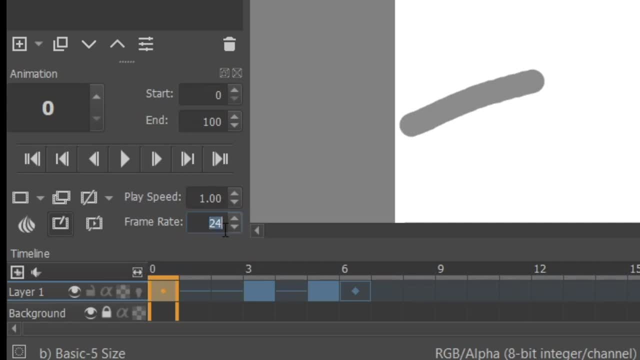 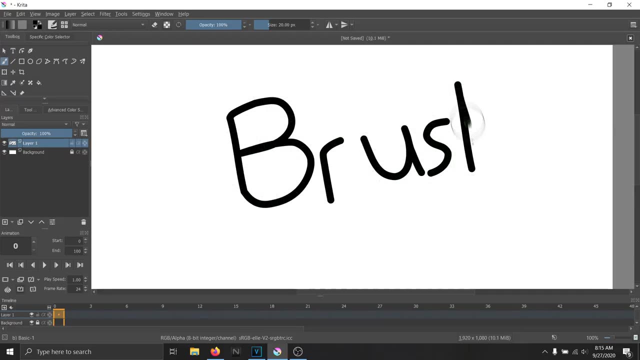 Going below 12 frames per second starts to get a little choppy. just so you know Choosing Brush and Brush Settings. Now I'm going to go over the Brush tool and its settings. The Brush tool is this little paintbrush under the toolbox tab. 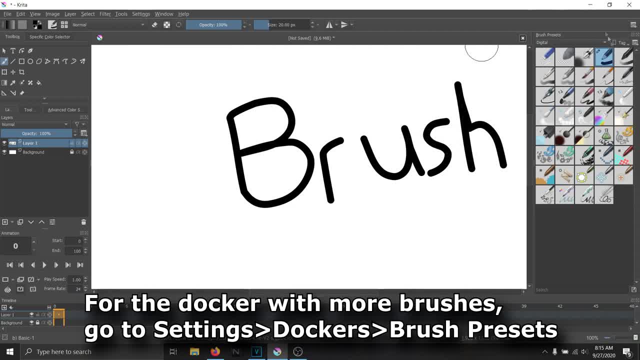 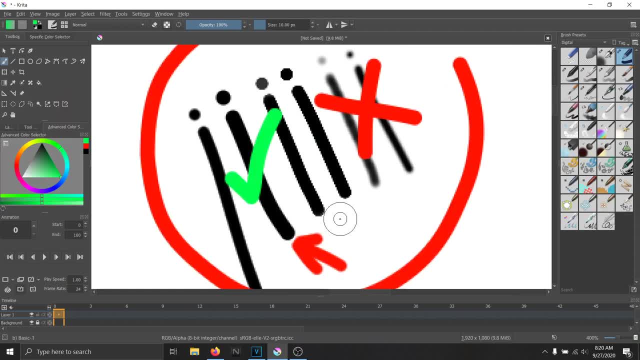 Krita comes with many brushes and you can add many more brushes for free For animations. you will want to choose a good circle brush that doesn't have too much of this transparent, anti-aliasing fuzziness stuff, but also not too jagged. 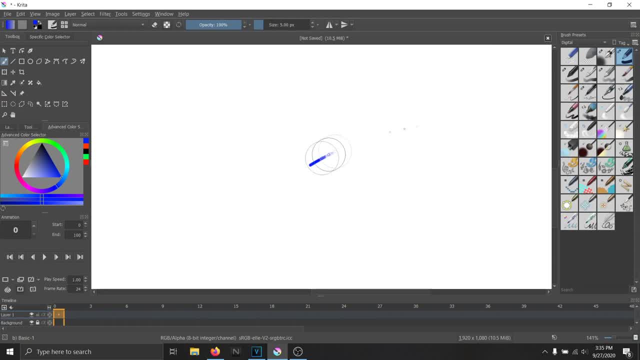 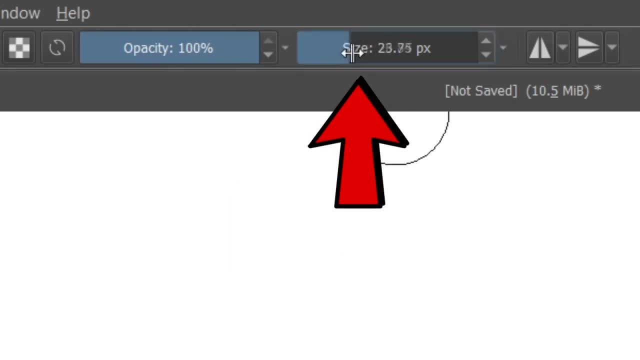 I find that the basic one brush works best for me and for my line art. For sizing your brushes, you can use the little bracket keys or go to the top and resize it by dragging it, Or you can press these little up and down arrows. 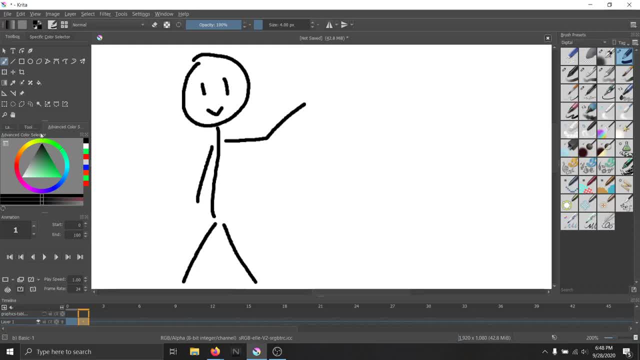 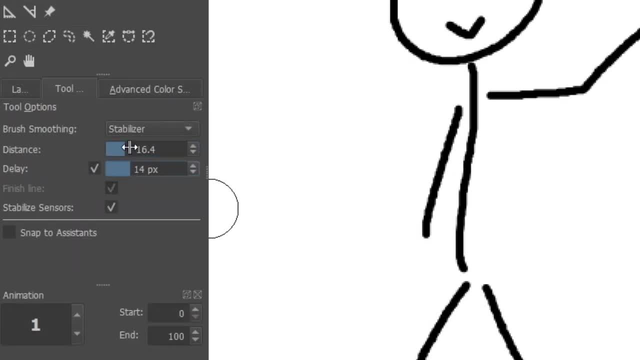 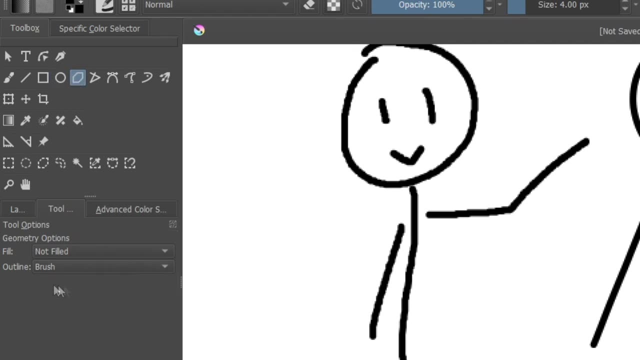 Now, if you don't own a drawing tablet and your mouse makes jagged lines, you can go to the Tool Options tab and select Stabilizer and play with the Distance and Delay settings till you're satisfied. Just as a side note, the Circle, Rectangle and Polygon tools also use the selected brush by default. 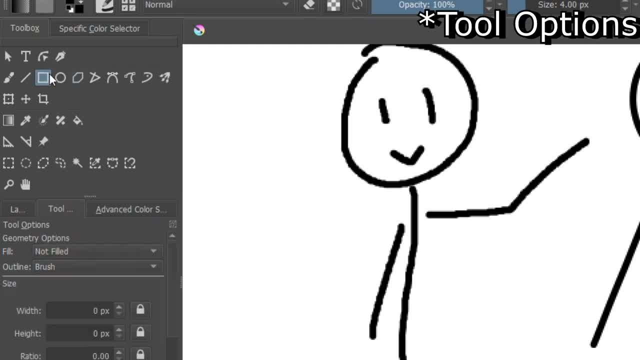 This can be changed by selecting the tool and going to the Tool Settings. Also, if you want to change the brush size, you can do that here. If you want your shape to be filled in, change the fill to background or foreground color, depending on what you want. 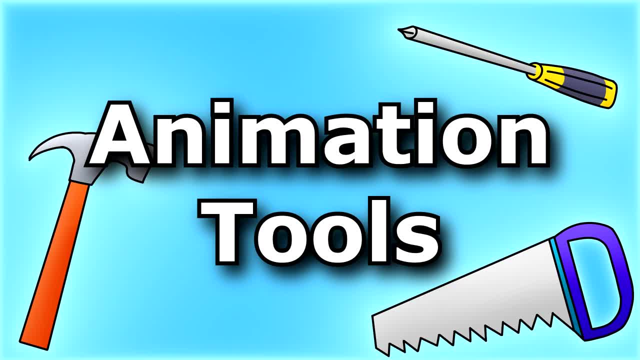 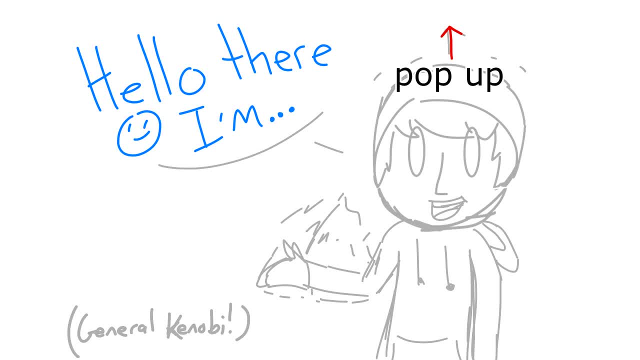 Recording Audio to Animate. Now that you have a basic knowledge of the tools and dockers for animating, you'll want something to animate too. And for this animation I'm going to be animating my character saying: Hello there, I'm Metro Animates. 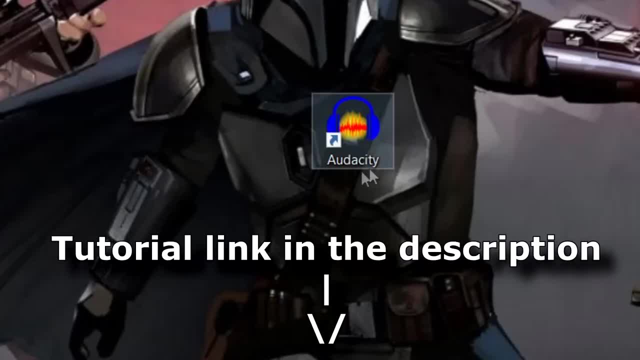 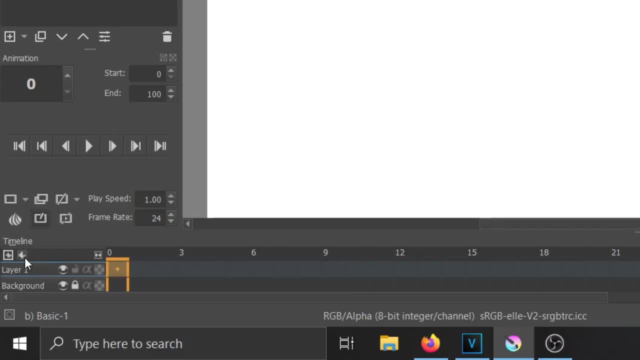 You can record this in any program you want, But I recommend Audacity, which is completely free and has everything you need to edit and record. To import the audio to your project, click on the little button on the bottom left corner and click on Open Audio and locate the audio file. 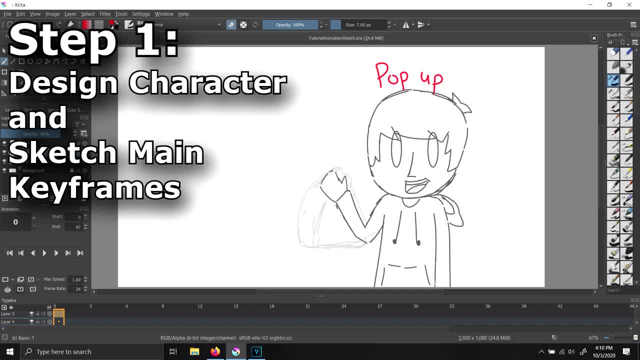 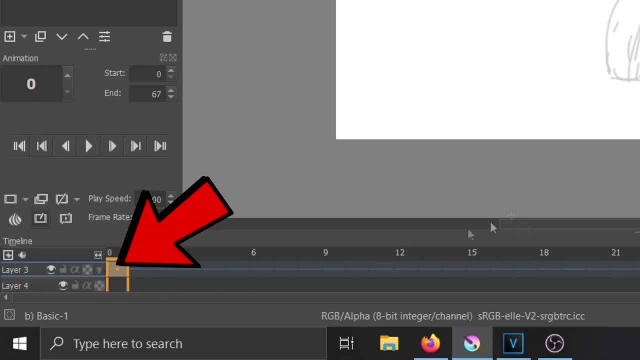 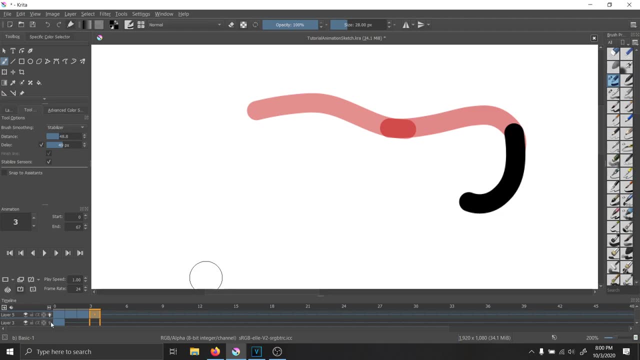 Sketching Your Character in Animation Frames. Now step one to animating is sketching out the main keyframes and design of your character. First step: turn on Onionskin by pressing on this little light bulb next to the timeline. This allows you to see what you've drawn before and after your current keyframe. 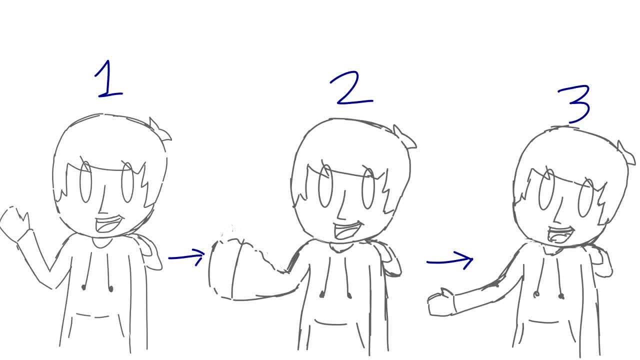 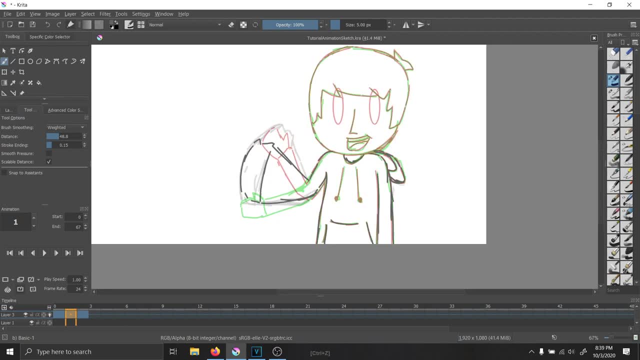 For my animation. I want my character to pop up and wave hello. Here I made a quick little time lapse of me sketching out my character. For the frames where my character pops up, I used the transform tool to move my character down. 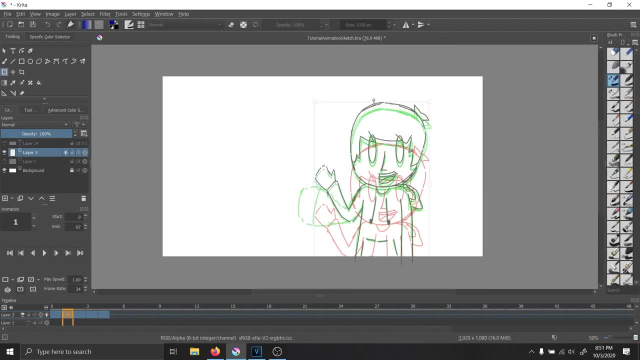 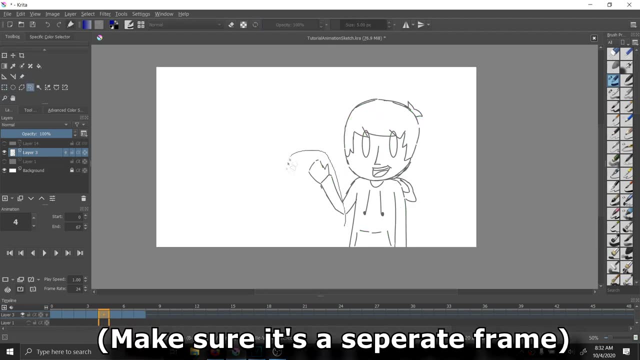 And on the next frame I stretched him out a little before he sits in his resting position to give him a little bit of a bounce. Also for the arm when it starts to move, I used the lasso tool and the transform tool to give it a smoother transition. before the in-between frame. 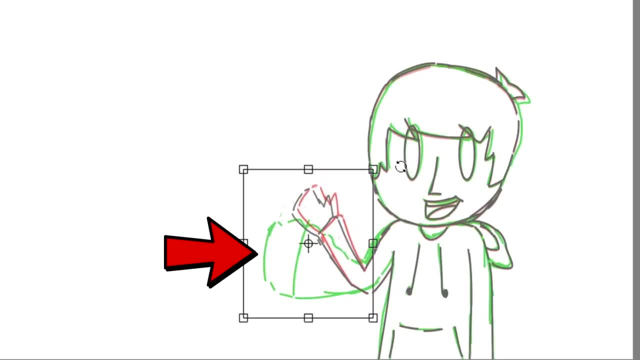 For the in-between for the arm, I used the lasso tool and the transform tool to give it a smoother transition before the in-between frame. For the in-between for the arm, I used the lasso tool and the transform tool to give it a smoother transition before the in-between frame. 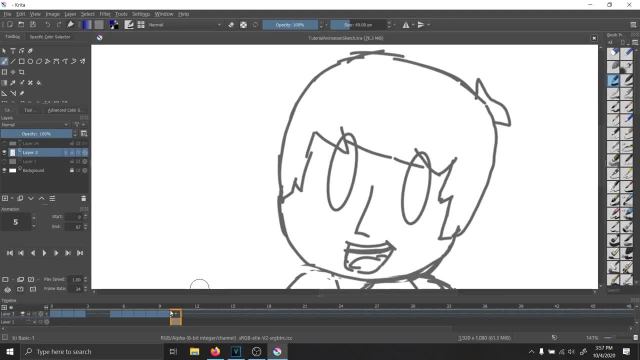 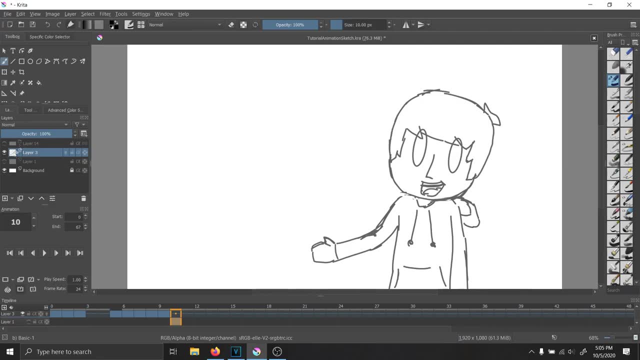 For a little more character, I'll add a bit of head movement when he waves Drawing your character's line art. The next step is drawing your line art to your sketched animation. so create a new layer for your line art. In fact, I would recommend creating two separate layers for the animated arm and head movement. 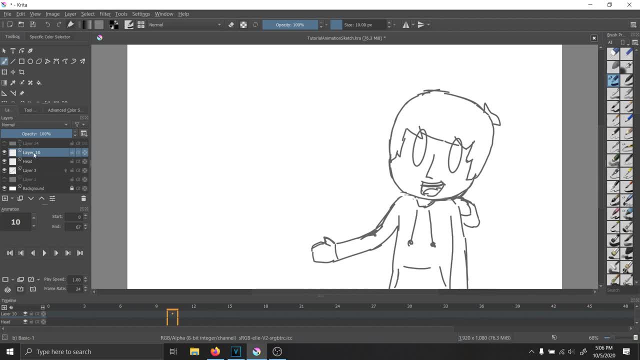 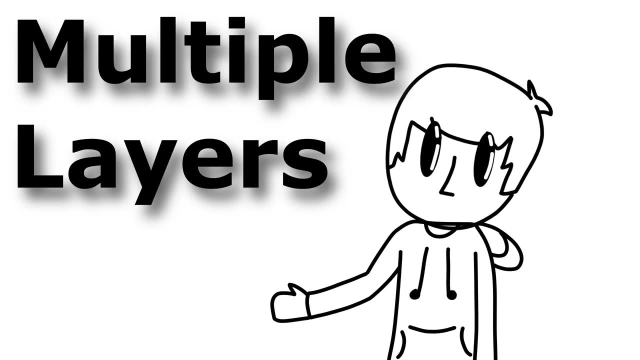 so we don't have to redraw the body every frame or worry about trying to erase the arms and head and head. Here's an example of animation with and without using multiple layers. Remember, you can use the transform tool to give a little extra bounce in life by 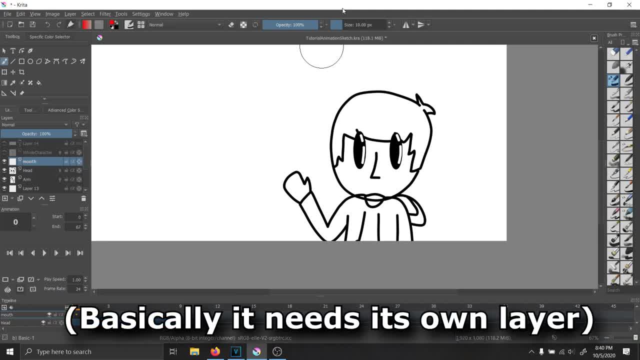 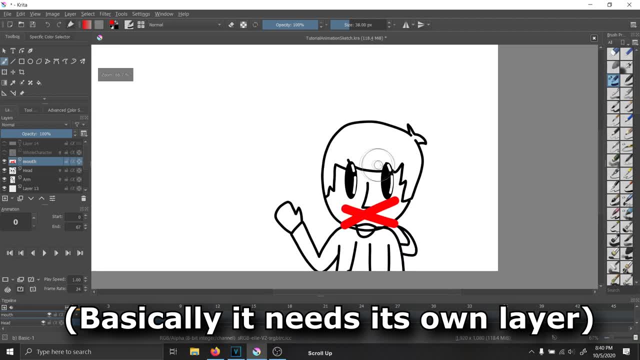 doing a little stretching, skewing or rotating. If you plan on lip syncing your character, I would recommend not drawing the mouth for now. Otherwise it'll be a lot of extra work of copying frames, erasing and redrawing, Coloring your 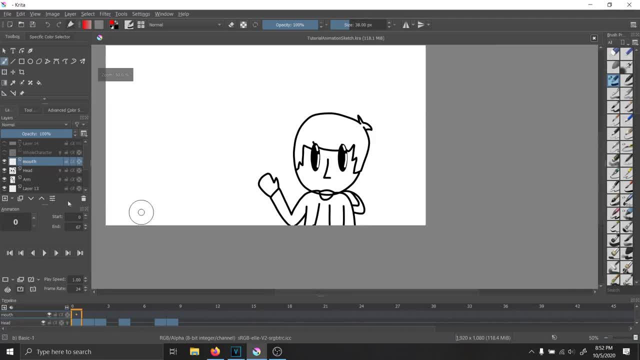 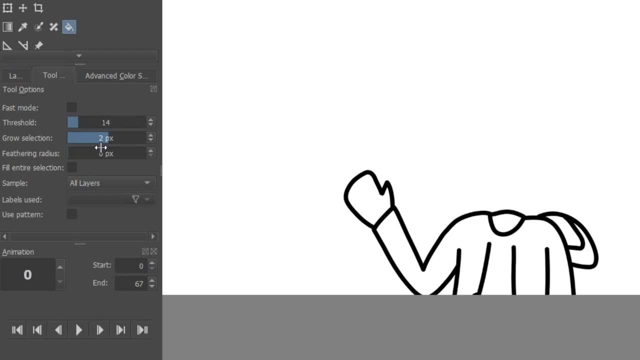 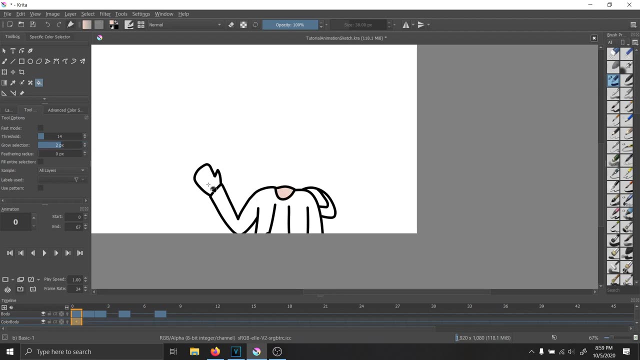 animations. For quickly coloring your animations in Krita: make a new layer and place it underneath the line art layers. using the up and down arrow buttons, You can take the fill tool and go to tool options and turn up the grow selection to two or three. Now just click inside your line art and it'll fill right in If 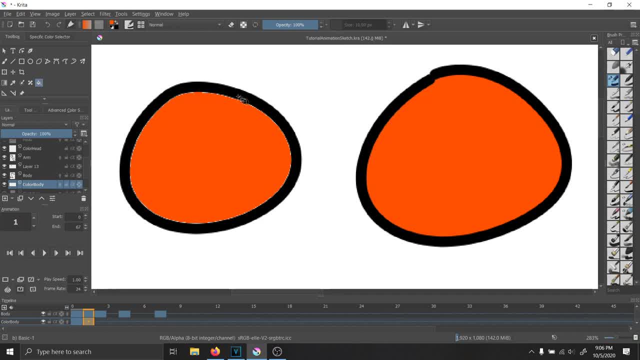 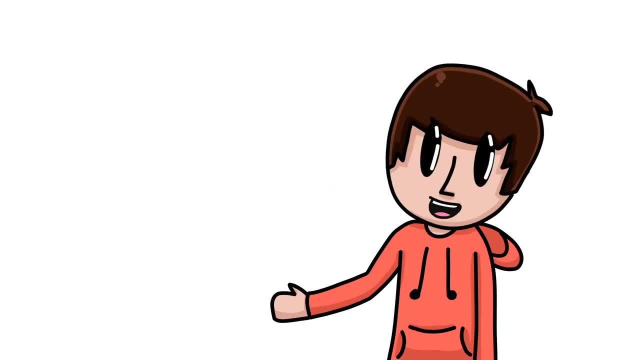 you didn't turn up the grow selection, it will turn out like this. Because Krita is a bitmap program, it uses pixels, not vector lines. For more complex animations, you can also use another separate layer for shading. That way you can use the 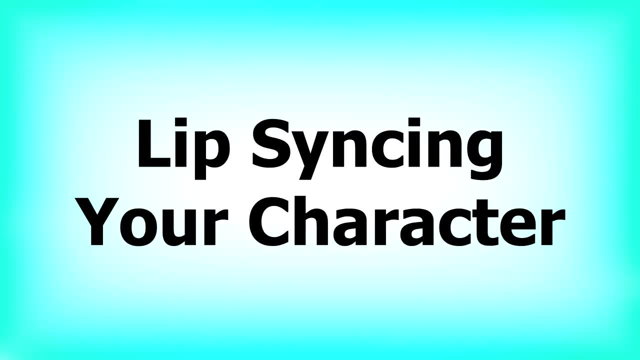 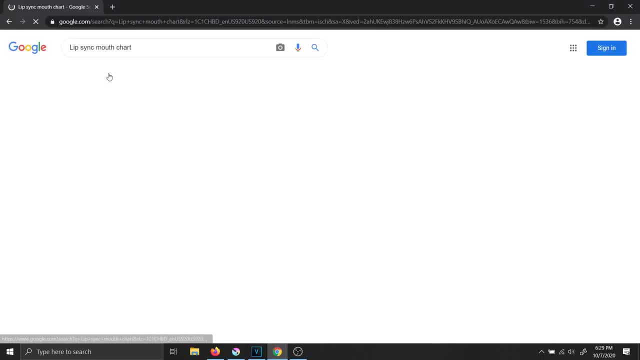 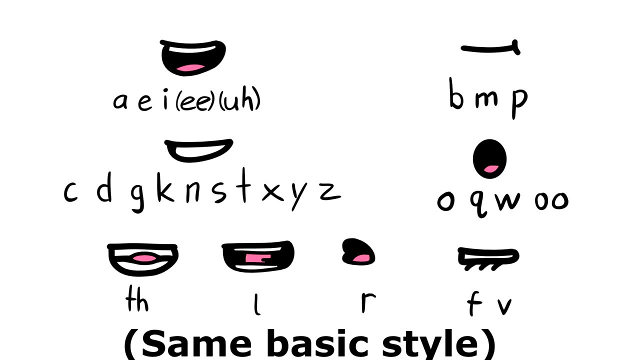 onion selection To create lip sync. I'd recommend first googling a good mouth chart example For this tutorial. I'll show you the mouse I use Now. if you want smooth looking lip sync, the two biggest tips I have are: keep each mouth the same style and keep